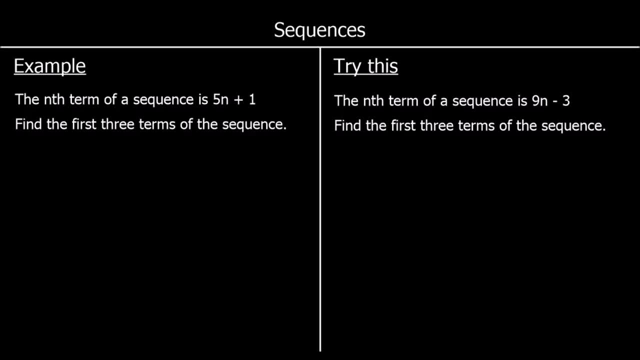 This question says the nth term of a sequence is 5n plus 1.. Find the first three terms of the sequence. So we call this 5n plus 1, the nth term is called the position to term rule. So if we substitute in the position we want, so the first position, which is 1,. 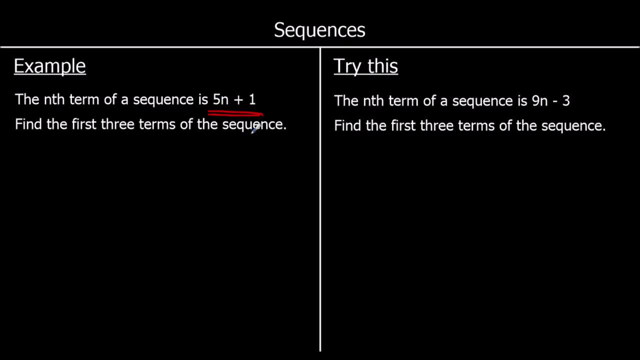 we'll get the first term. So if n is 1, what is 5n plus 1 worth? 5 times 1 is 5, plus 1 is 6.. Then if we want the second term, we substitute in: n is 2.. 5 times 2 is 10, plus 1 is 11.. 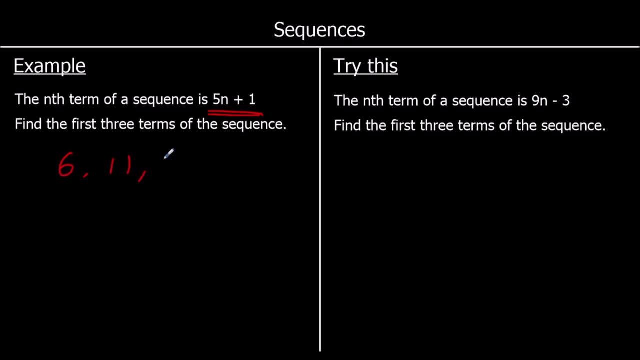 If we want the third term, we substitute in n is 3.. So 5, times 3 is 15, plus 1 is 16.. And we can find any term using this method. So if we want the 100th, 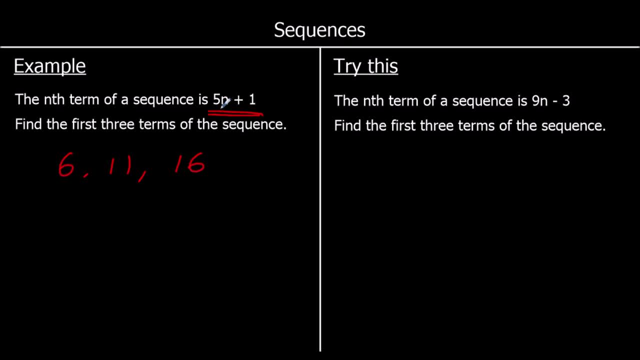 term, it'll be 5 times 100, 500, plus 1, 501.. But these are the first three terms. so that's our answer. There's one for you to try here. So find the first three terms of this sequence. 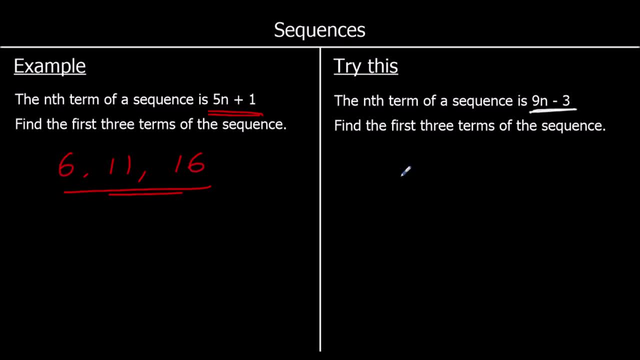 To find the first term we are going to substitute in: n is 1.. So that'd be 9 times 1, which is 9, take away 3, which is 6.. For the second term, n is 2.. So 9 twos are 18,. 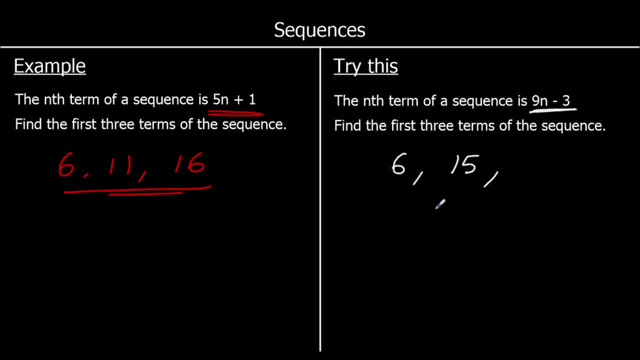 take away 3 is 15.. And the third term, 9. threes are 27,. take away 3, is 24.. So those are the first three terms. This question says the nth term of a sequence is 3n minus 5.. Is 95 in the sequence? 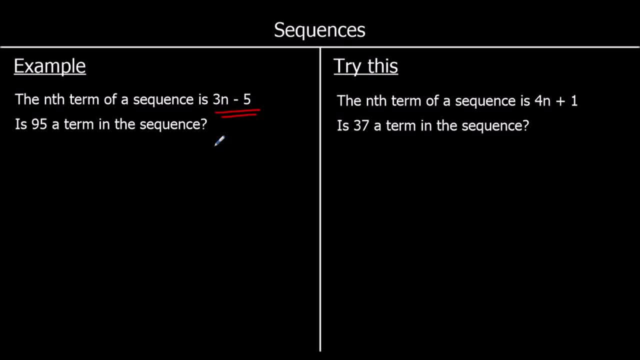 So is 95 a term in this sequence. So what we can do is we can try and find out what 95, what term 95 is. So if we solve 3n minus 5 equals 95, the answer will be what term 95 is in the sequence. So what value of n would make? 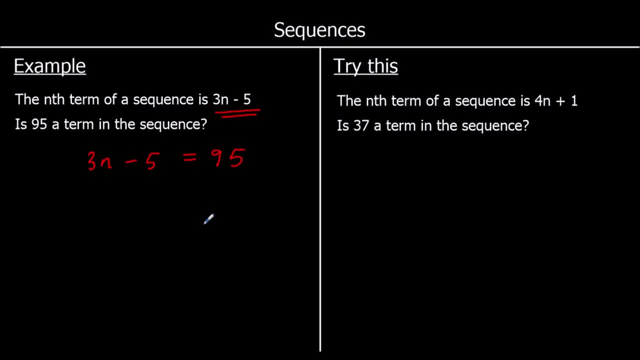 this sequence 95?? So that's plus 5 to both sides. So 3n is 100.. And then divide both sides by 3.. Well, 100 over 3 is 33.3 recurring, And we don't have a 33.3 recurring term in a sequence, So it's not in the sequence. 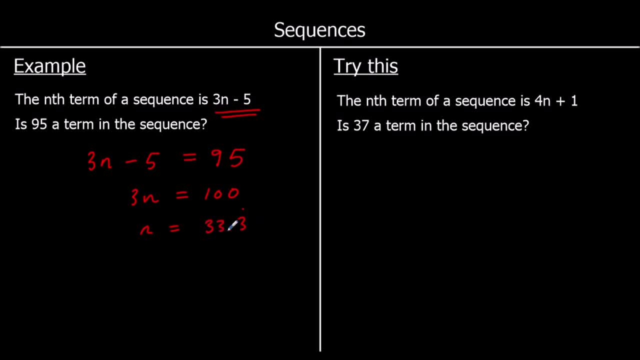 So the 33rd term would be too small And then the 34th term would be too big. So it's not in the sequence. It's not in the sequence because this isn't a whole number. We could have also answered this question by finding the 33rd term. 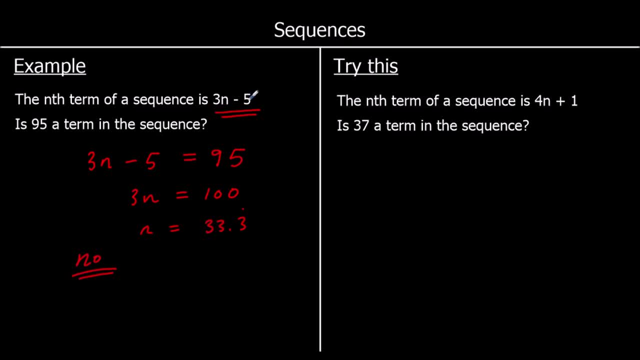 So 3, 33 is a 99, minus 5 is 94. So we could have said: the 33rd term is 94. The 34th term will be 97. So three 34s are 102.. Take away: 5 is 97. Or you could just know it's going up in. 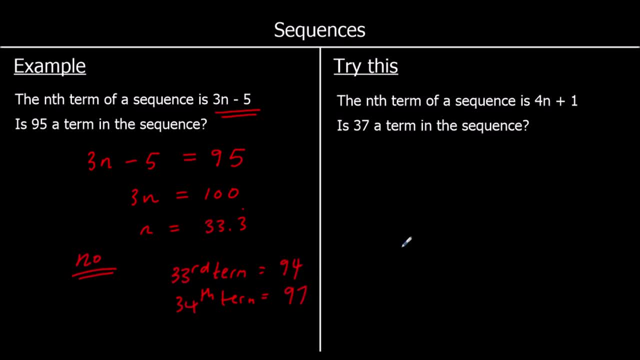 3s every time and add on 3 to the 33rd term, And 95 is in between these two, So it's not in the sequence. It doesn't matter which of the methods you use, as long as you prove. 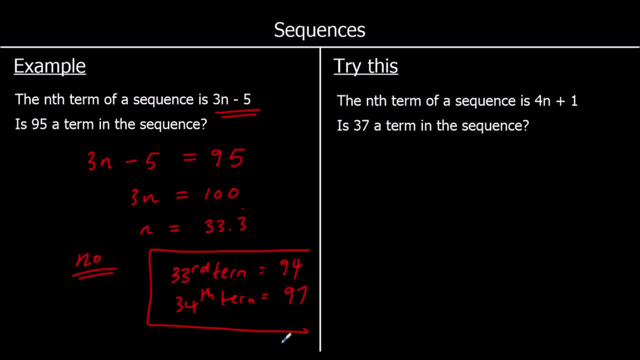 you show it's not in the sequence. Okay, one for you to try, So give this a go. The nth term of a sequence is 4n plus 1, is 37 a term in the sequence. So if it is in the sequence, 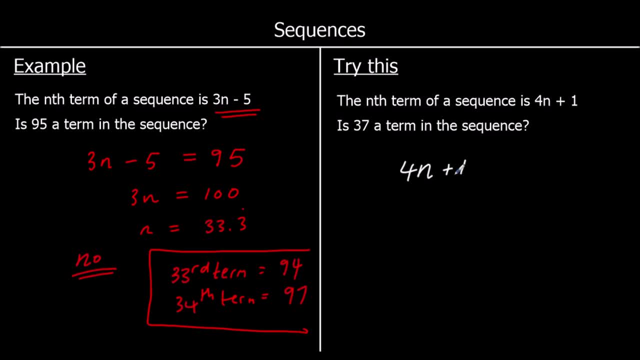 there will be a number that makes 4 n plus 1 equal to 37. So if 37 is in the sequence, there will be a number that makes 4n plus 1 equal to 37. So if we try and solve this, let's take 1 away from both sides. 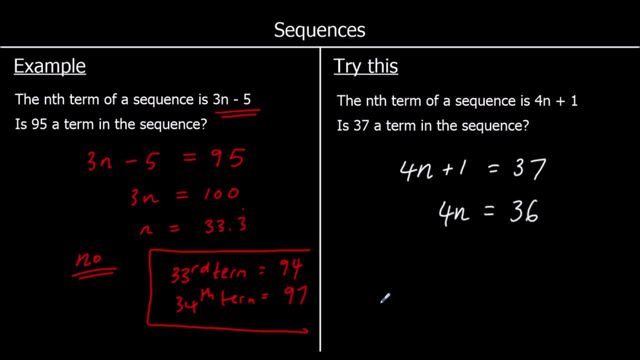 So 4n equals 36.. And then divide both sides by 4. And what we get n is 9.. So it is in the sequence It's the ninth term: 4 times 9 is 36, plus 1 is 37.. 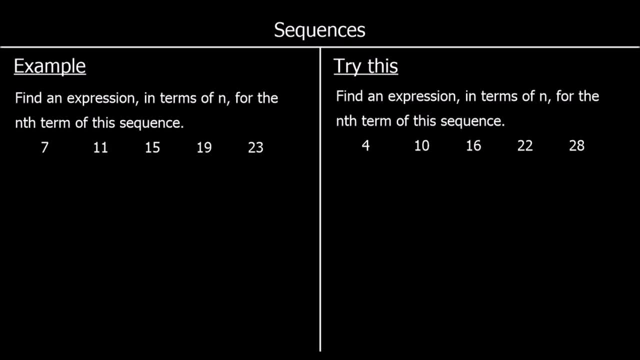 So it's the ninth term. This question has given us the sequence And it says: find an expression in terms of n for the nth term of the sequence. So we need to find the nth term this time. So let's look at the sequence. 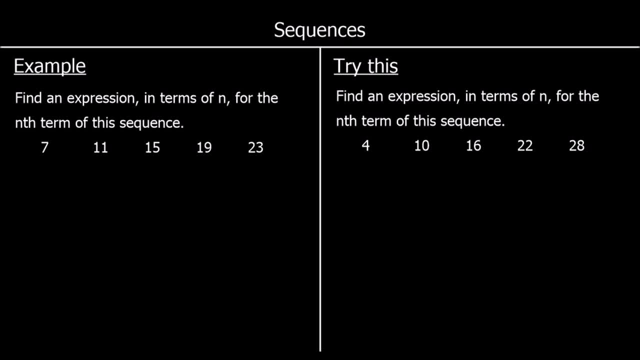 And let's look at what it's going up in, So we can see from 7 to 11.. From 11 to 15.. From 15 to 19.. From 19.. From 17 to 23.. It's going up in 4s every time. 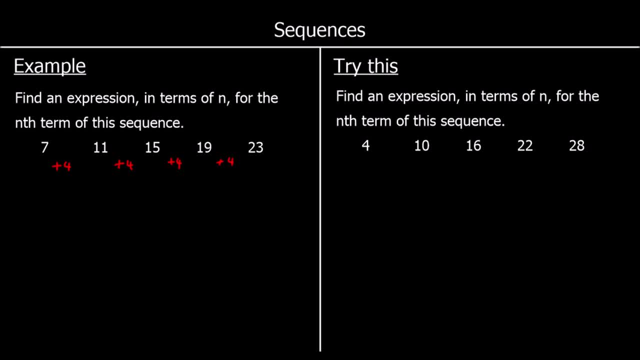 That tells us it's 4n, It's 4n And 4n is the 4 times table. 1, 4 is 4.. 2, 4 is 8.. 3, 4 is 12.. 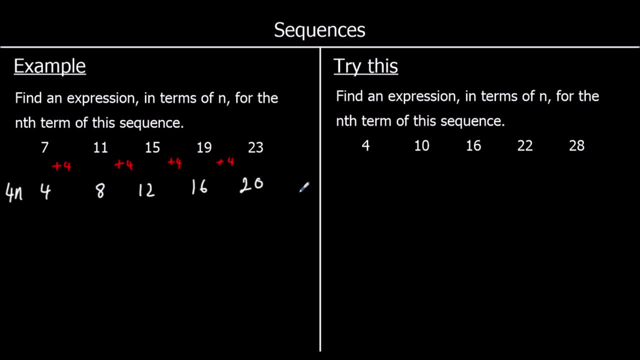 4, 4 is 16. And 5, 4 is 20.. So this sequence isn't the 4 times table, But what we can see is it's always 3 more than the 4 times table. 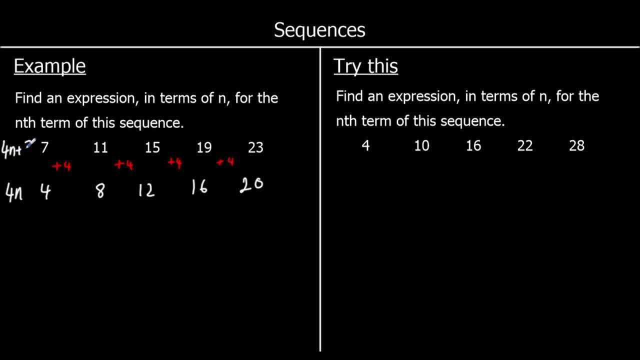 So our sequence is called 4n plus 3.. So it's always 3 more than the 4 times table. Okay, one for you to try, So give this one a go. So we've got 4,, 10,, 16,, 22,, 28.. 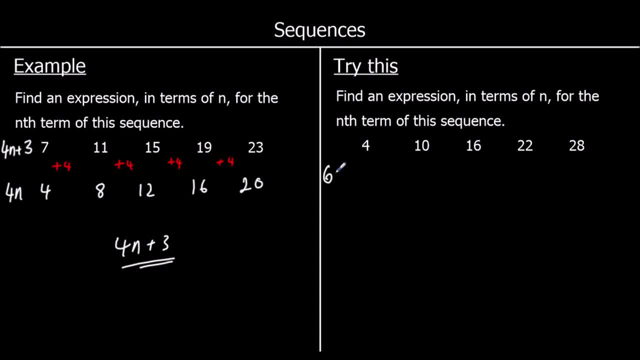 And you can see it's going up in 6s, So it's going to be 6n this time. So the 6 times table: 6, 12,, 18,, 24,, 30. Our sequence is like the 6 times table. 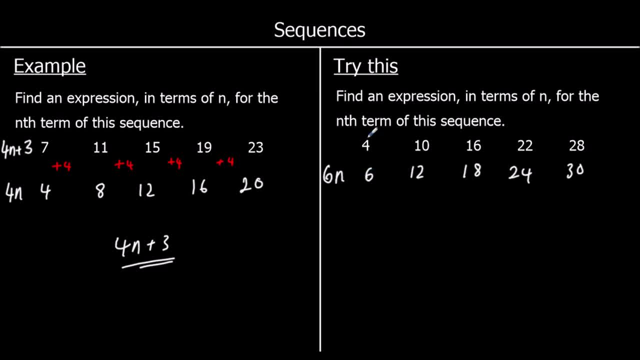 But it's not the 6 times table. It's always 2 less than the 6 times table, So it's the 6 times table. take away 2.. Here's another example. This time we can see the number 2,. 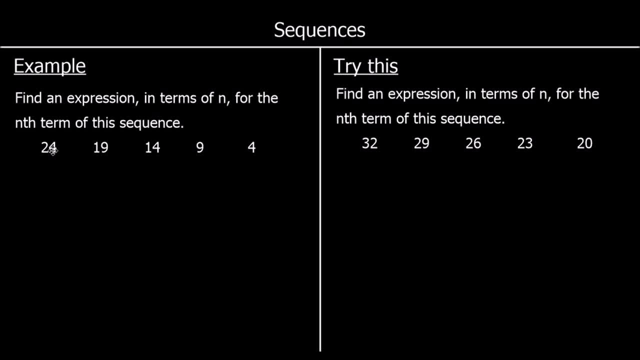 and the numbers are going down. They're getting smaller every time. So the difference between the terms, the term to term rule, is minus 5 this time. So we're going down by 5 every time. So we're going to say it's minus 5n. 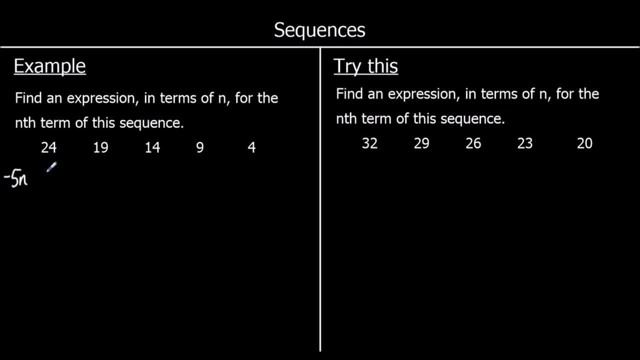 So it's the minus 5, the negative 5 times table. So that's negative 5 times 1, is negative 5.. Negative 5 times 2 is negative 10.. 3 negative 5 times 2 is negative 10.. 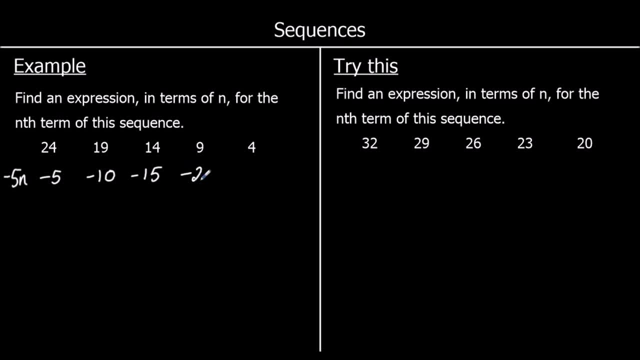 3 negative 5 times 2 is negative 10.. 3 negative 5 times 2 is negative 15. And so on. So we've got the negative 5 times table. And what do we have to do to the negative 5 times table? 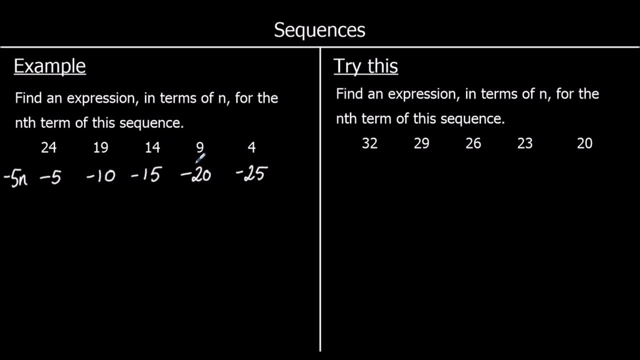 to get our sequence, So we need to add on 29.. So we're going to say it's minus 5n plus 29.. You could also write it the other way round and say it's 29 minus 5n. You could also write it the other way round and say it's 29 minus 5n. 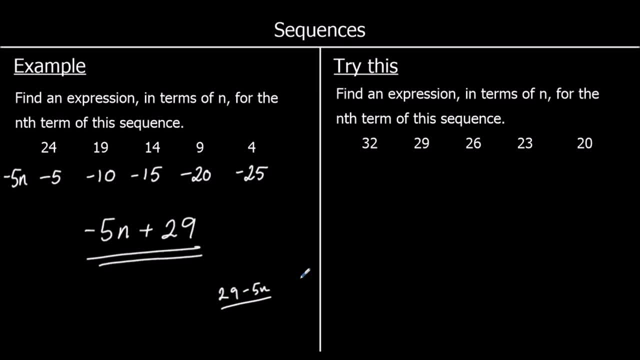 Either way, it doesn't matter. Okay, one for you to try, So give this one a go. So let's look for the term to term rule And we can see that this sequence is going down by 3 every time. So if it goes down by 3 every time, 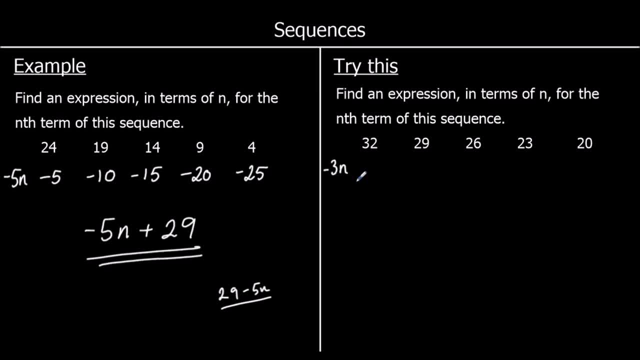 we're going to say it's minus 3n, It's the negative 3 times table. So that goes negative 3, negative 6, negative 9, negative 12, negative 15.. What do we have to do to the negative 3 times table? 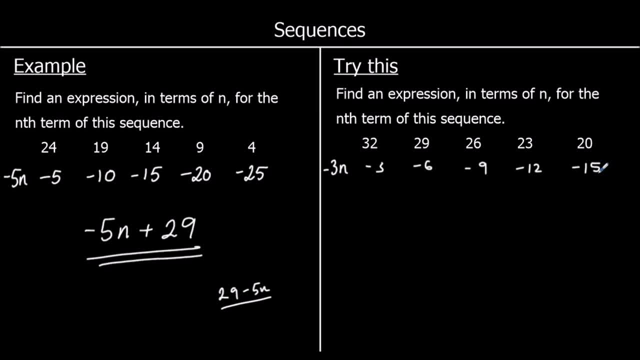 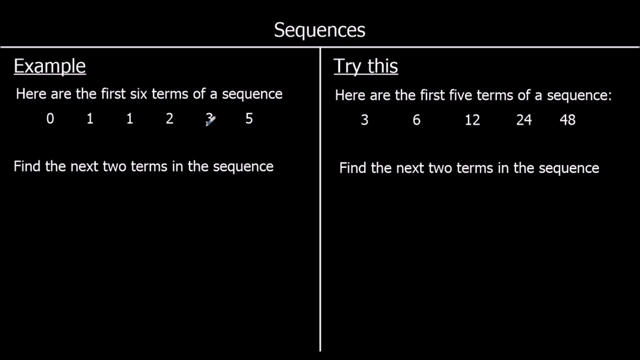 to get our sequence, What do we have to add on to it? We have to add on 35. So it's the negative 3 times table plus 35. And here are some different sequences. are some different sequences. we've got the first six terms of a sequence and we're being asked for. 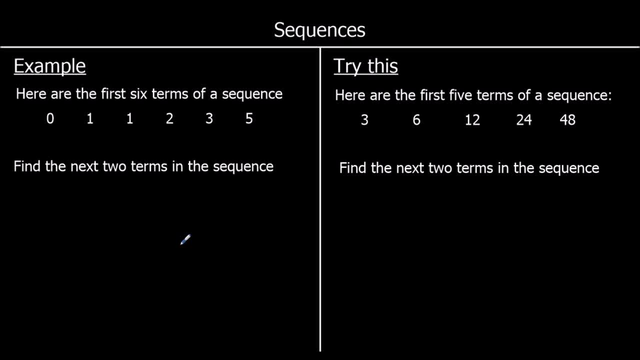 the next two terms. so this is a fibonacci sequence, so this is a sequence that you need to be aware of. so the first two terms add to make the third term. the second and third terms add to make the fourth term. the third and fourth term add to make the fifth term. 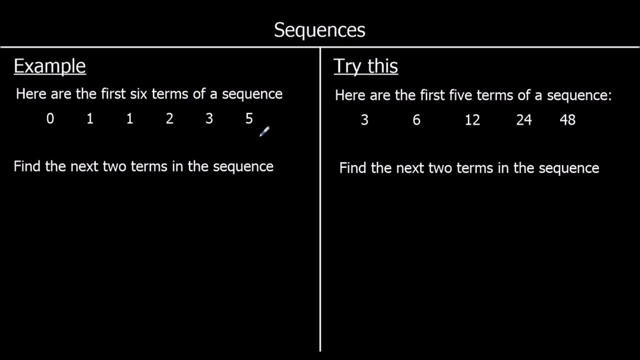 the fourth and fifth terms add to make the sixth term. so the fifth and sixth term add to make the seventh term. so three and five make eight, and then five and eight are going to add for the next one. five plus eight is thirteen, and we could keep going if we wanted. 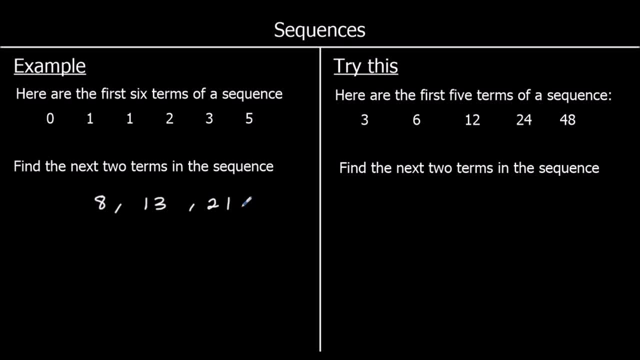 so the next time will be eight plus 13, which be 21 and 13 plus 21. but we only needed the next two terms. so this is a fibonacci sequence and the previous two terms add to make the next term. here's a different sequence, so try and figure out the next two terms of this sequence. 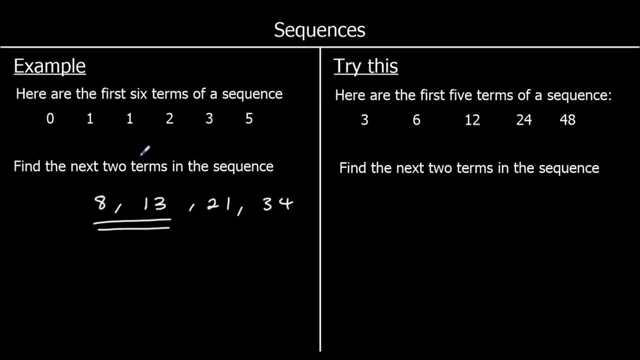 and this sequence is called a geometric sequence. so we multiply by something every time. so in this sequence we're doubling the previous term to go from one term to the next term, we multiply by two, so the next term is going to be 248, which is 96, and then we're going to have two 96s. 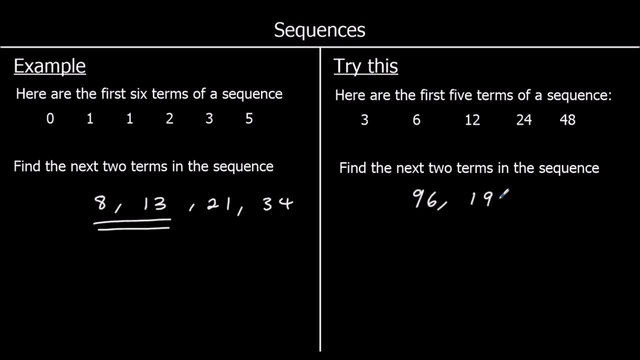 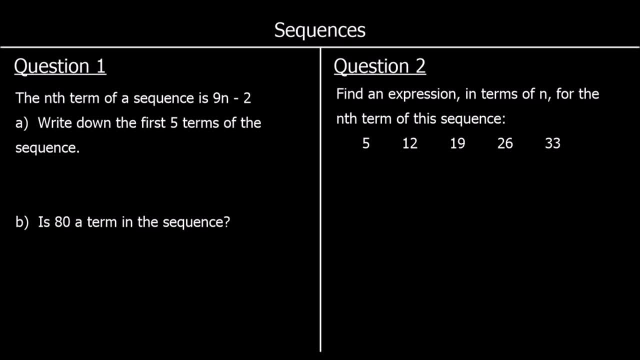 which will be 100 and 92.. so to finish up, we've got two questions. pause the video, give them a go and press play when you're ready for the answers. question one says the nth term of a sequence is 9n minus 2.. write down the first. 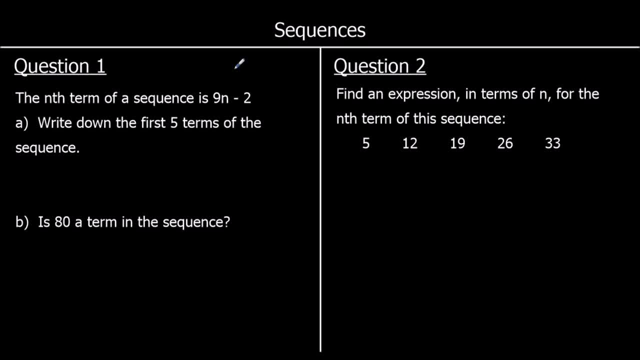 five terms of the sequence. so 9n minus 2 is our nth term. so if we substitute one in we find the first term. so 9 times 1 is 10, j, 2,3. is 9 and 3 is 11. 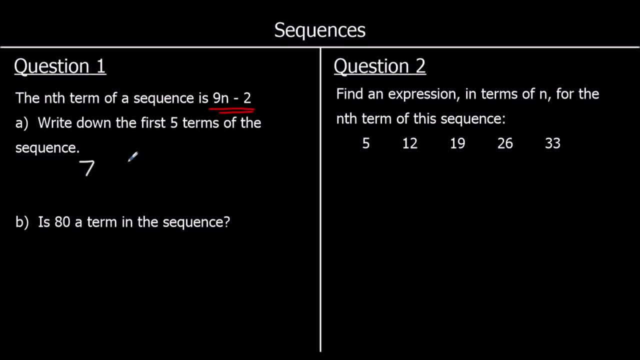 j 2 is 7 and 4 is 11. j 2 is 9 and 3 is 9, j 2 is 9 and 3 is 13 y j 2 is 13. n plus 5 is 3, 1 minus 2 is 7. 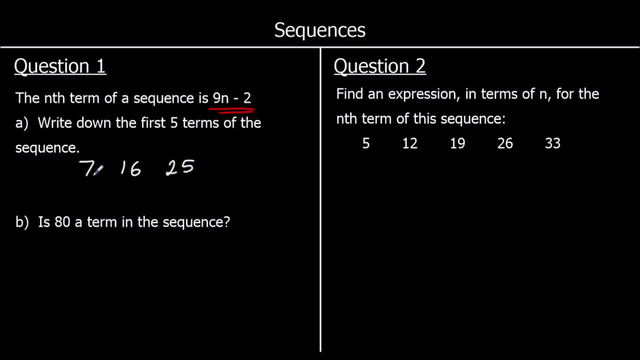 um, when calculating y, we calculate 2 into this, and 7 times 2 is 22.. and 7 times 2 times 23.. going up in 9 every time, so we can add on 9, and then add on 9 again to find the next. 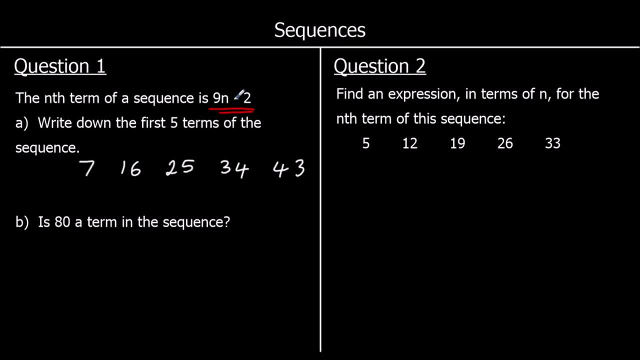 two terms And we can check our answer: 9 fives for the fifth term is 45, take away 2, 43. Part B says is 80 a term in the sequence. So if 80 is in the sequence there will be. 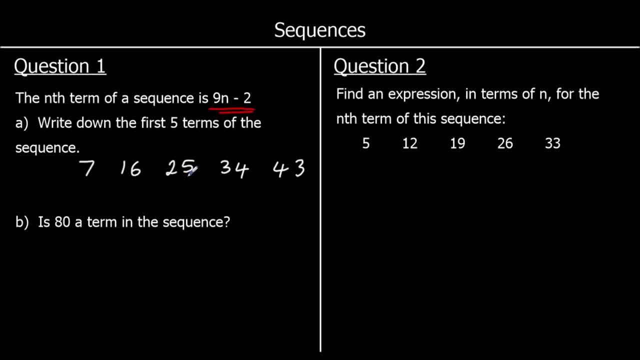 a whole number that makes 9n minus 2 equal to 80.. So we can try and solve this, and if the answer is a whole number, then it is in the sequence. So let's plus 2 to both sides, so 9n is equal to 82, and then divide both sides by 9,, so n is 82. 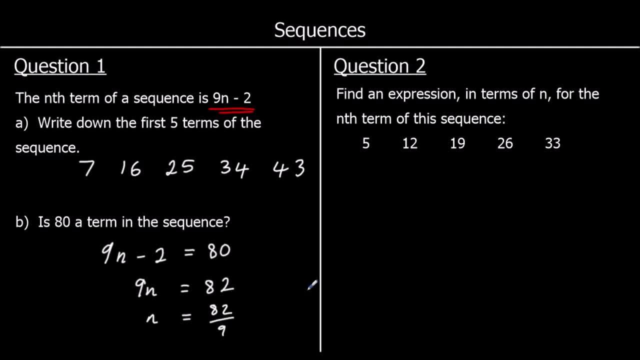 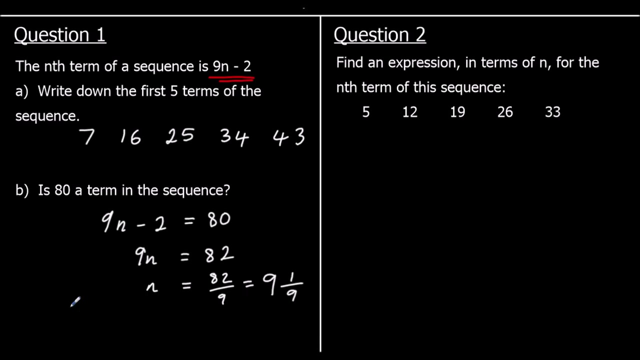 82 is not in the 9 times table. this isn't a whole number. 82 is well, 9 nines make 81, so we've got 9 whole ones and 1 ninth. So 80 is not in the sequence, it is in between. 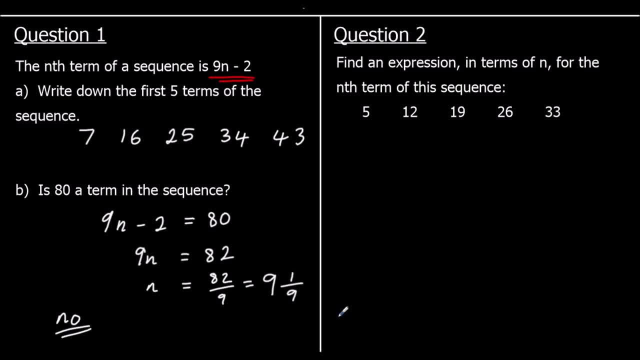 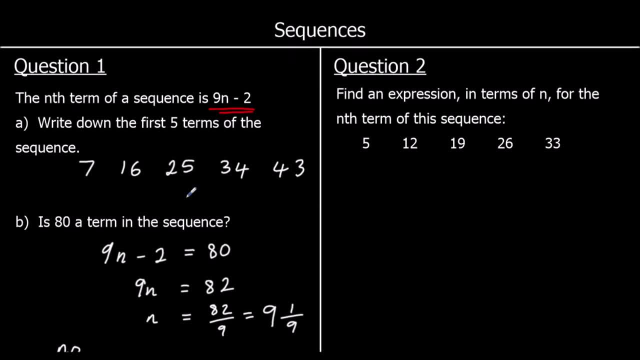 the ninth and the tenth terms. Question 2, find an expression in terms of n for the nth term of this sequence. So we've got 5,, 12,, 19,, 26,, 33.. So let's look for the term-to-term rule. What is the sequence going? 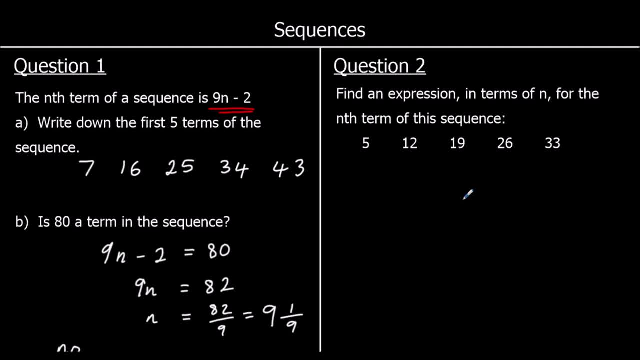 up in. So this sequence is going up by 7 each time. so we can say it's 7n and 7n is the 7th term. 7 times table, that's 7,, 14,, 21,, 28,, 35. So what do we have to do to the 7 times table?